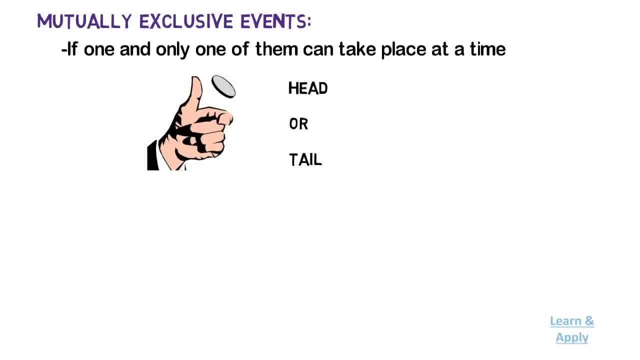 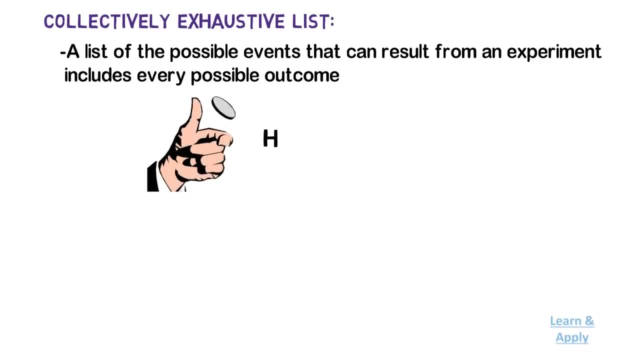 In our example of tossing a coin, only head or tail can occur. Collectively exhaustive list. When a list of the possible events that can result from an experiment includes every possible outcome, the list is said to be collectively exhaustive. In our example, the list head and tail is collectively exhaustive. 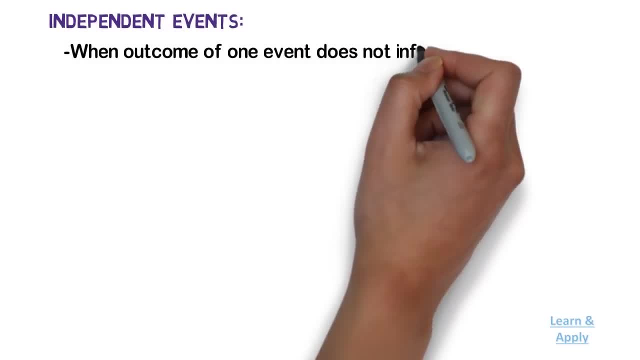 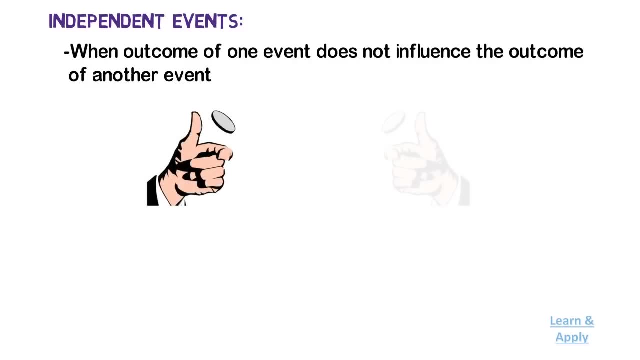 Independent events. When outcome of one event does not influence the outcome of another event, the two events are called as independent events. In our example, the outcome of first tossing and second tossing are independent Types of distribution. There are too many types of distribution of data. 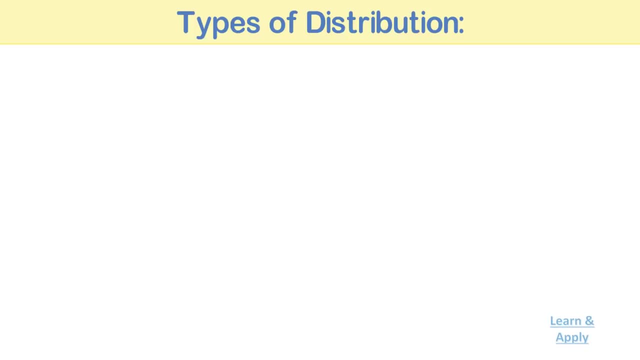 But we are focusing on mainly five types of distribution: 1. Binomial distribution, 2. Poisson distribution, 3. Exponential distribution, 4. Weibull distribution, 5. Poisson distribution And, the most important, 5. Normal distribution. 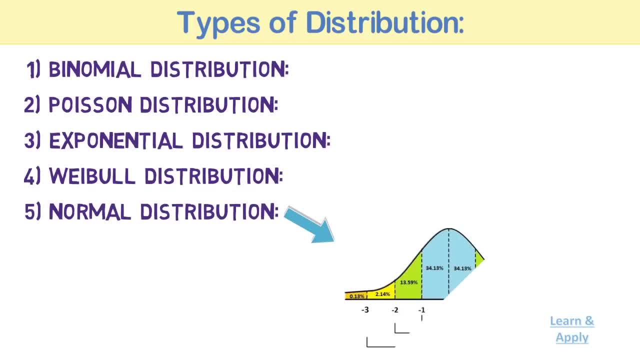 I have already explained normal distribution in very detail during study of histogram, But it's worth to see it again. Out of these five distributions, binomial and Poisson distribution are for discrete variables, Whereas remaining three are for continuous variable. I will explain distributions for discrete variables in this video. 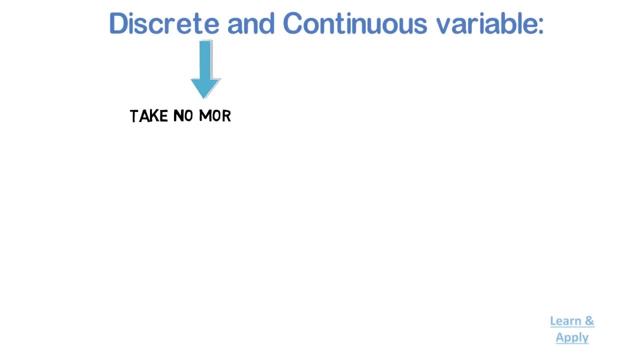 Discrete and continuous variable. Variable is discrete if it can take no more than countable number of values, For example, the number of defective atoms in a sample of 20 atoms. Variable is continuous if it can take any value in the interval. 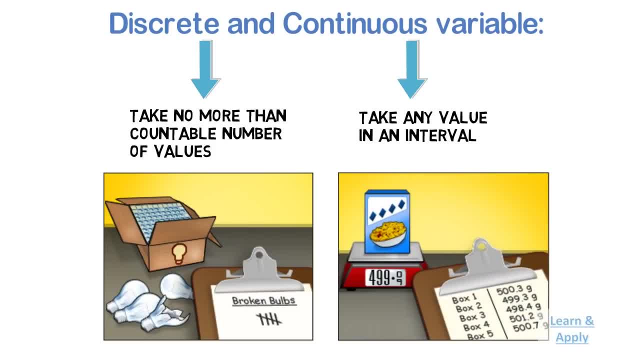 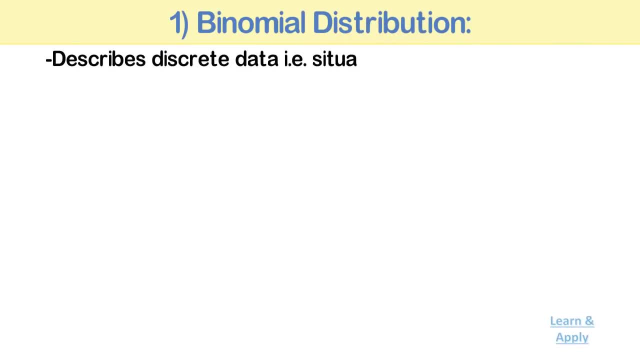 For example, the weights from a couple of 20 cereal boxes. 1. Binomial distribution: The binomial distribution describes discrete data situations where there can be only two results in a random experiment. The binomial distribution describes discrete data situations where there can be only two results in a random experiment. 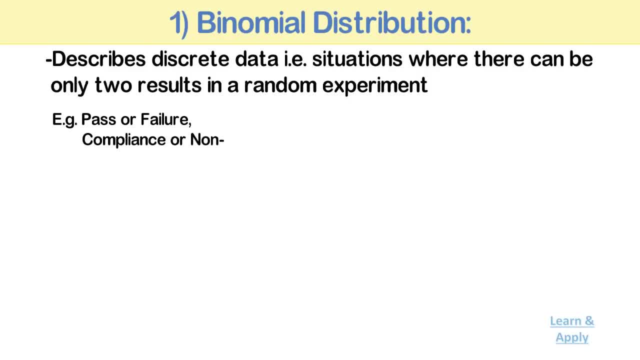 Examples are: Pass or Failure, Compliance or Non-compliance, Yes or No, Measures of central tendency and dispersion. For the binomial distribution, P is equal to probability of success, Q is equal to probability of failure and which is equal to 1-P. 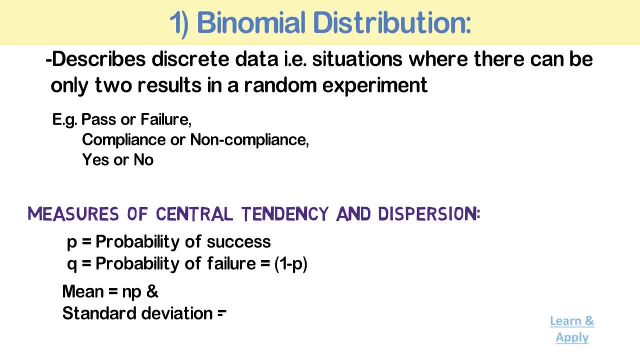 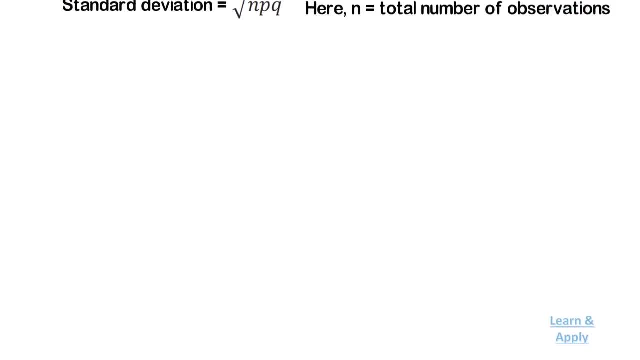 Mean is equal to n into P and standard deviation which is equal to square root of nP cube. Here n is the total number of observations. Let x be a binomial random variable, Then its probability mass function is P, P, P, P, P. 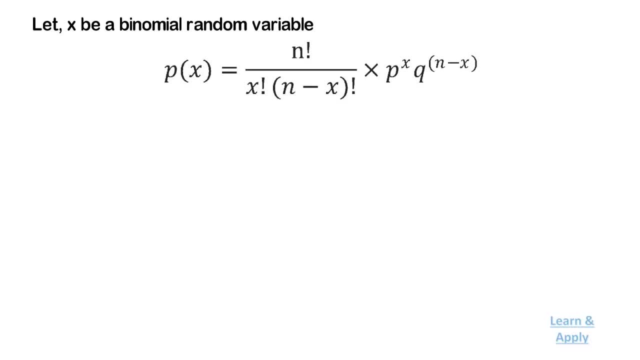 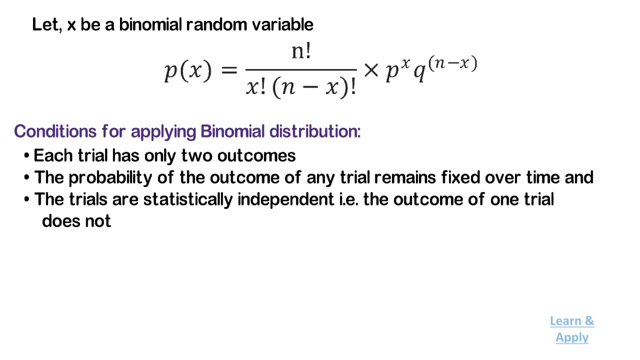 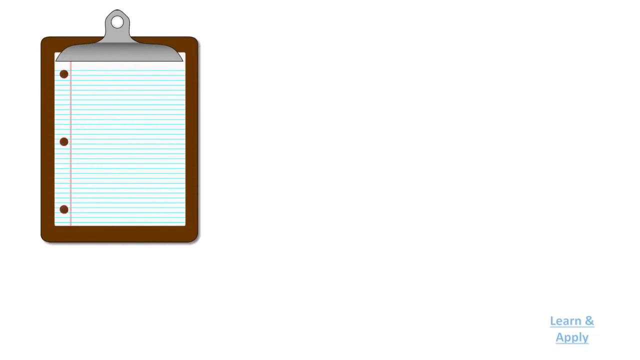 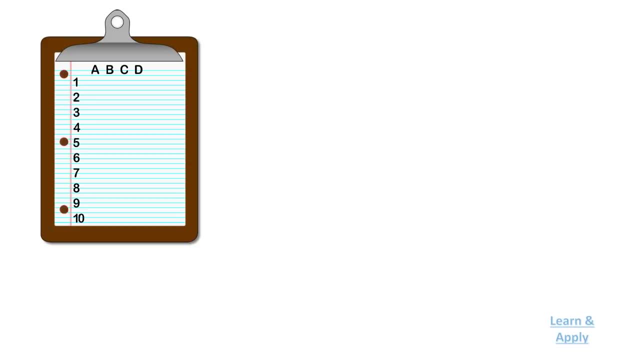 choices for each question, only one of which is correct. Suppose a student is to select the answer for every question randomly. Let x be the number of questions the student answers correctly. Then x has a binomial distribution with parameters: n is equal to 10 and p is equal to 1 by 4,. 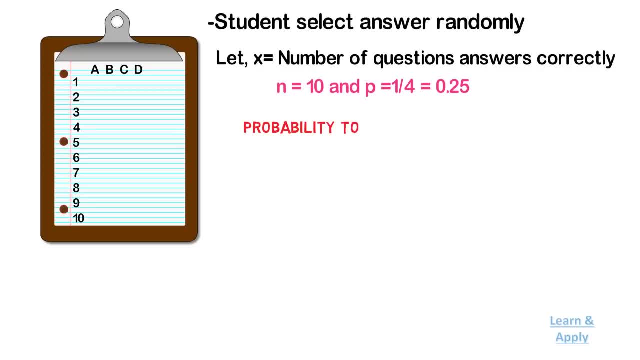 that is 0.25.. Now what is the probability for the student to get no answer correct Here? x is equal to 0. So probability of 0, which is equal to 10, factorial into 0.25, raise to 0 into bracket 1 minus. 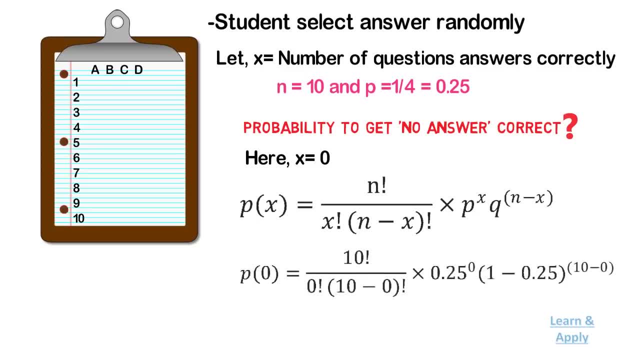 0.25 raise to 10 minus 0 whole, divided by 0 factorial, into 10 minus 0 factorial, Which is equal to 0.0563.. That is 5.63. is the probability that no answer will be correct. 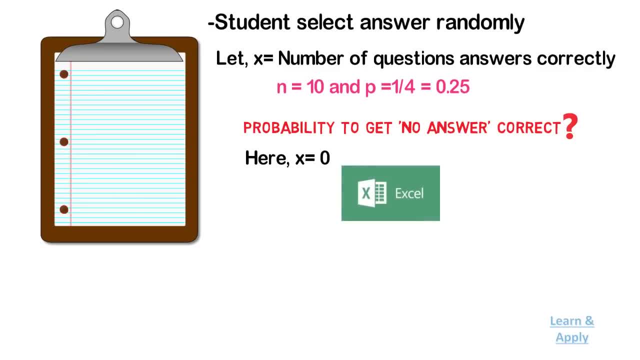 We can also use excel to find probability related to binomial distribution random variable: the number of successes x in the n trials, And it is calculated as probability which is equal to binom dist x, n, p and 0.. For above example, probability which is equal to binom dist x, n, p and 0. 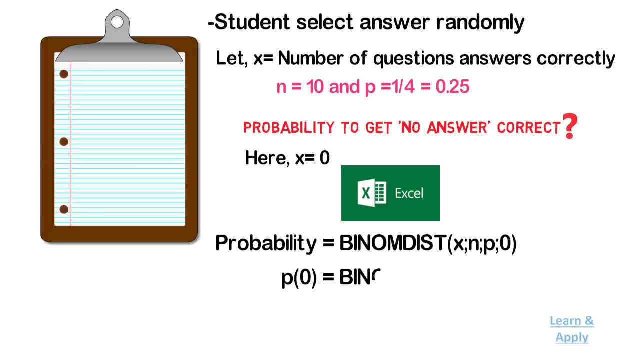 For above example, probability which is equal to binom dist x, n, p and 0.. For above example, probability which is equal to binom dist x, n, p and 0.. The normalized number ofgeme �ät 자� equal to p, nm, xy. 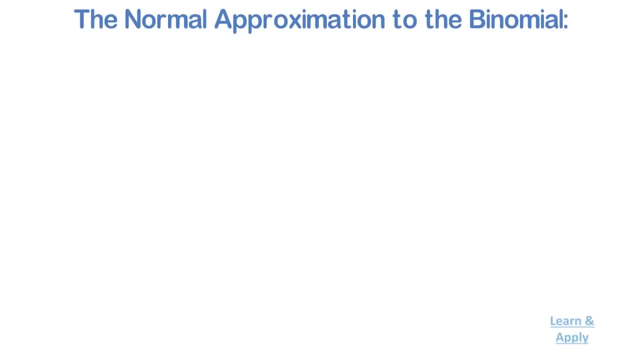 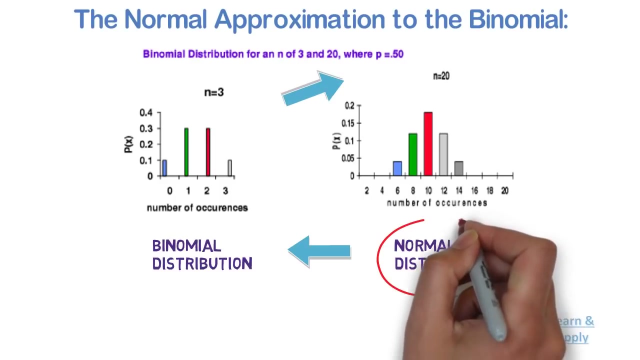 The normal approximation to the binomial using the normal distribution. A continuous distribution as a substitute for binomial distribution, that is, a discrete distribution for large values of n, Seems reasonable. Nos. colonial values When increases, a binomial distribution gets closer and closer to a normal distribution. 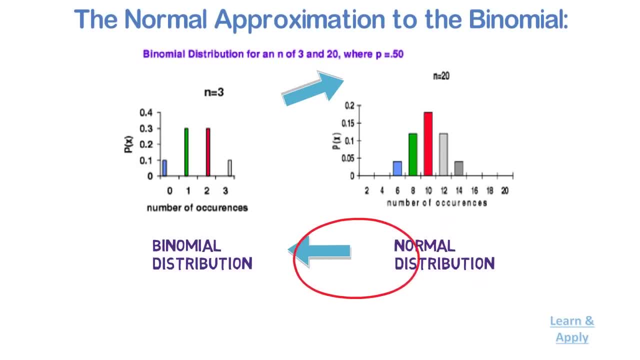 The normal probability distribution is generally deemed a good approximation to the binomial probability distribution when np and n into 1-p are both greater than 5. That is, p is equal to 0.5, then n should be greater than or equal to 10.. 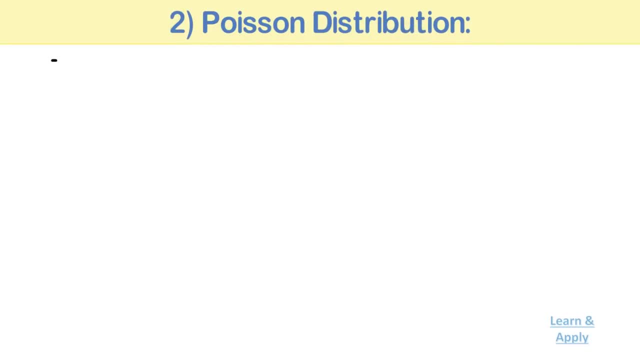 2. Poisson distribution. Poisson distribution also describes discrete data, that is, situations where the random variable can take integer values. For example, number of patients arriving at a physician's office, number of cars arriving at a toll booth. measures of central tendency and dispersion. 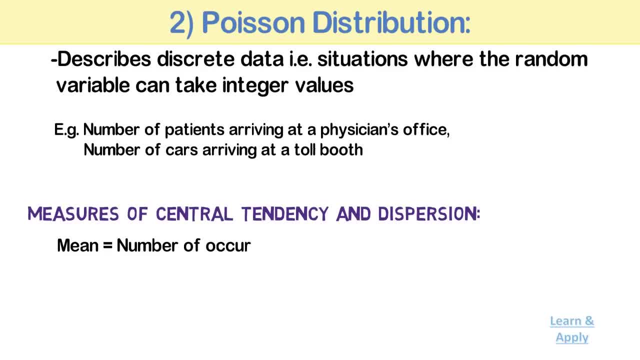 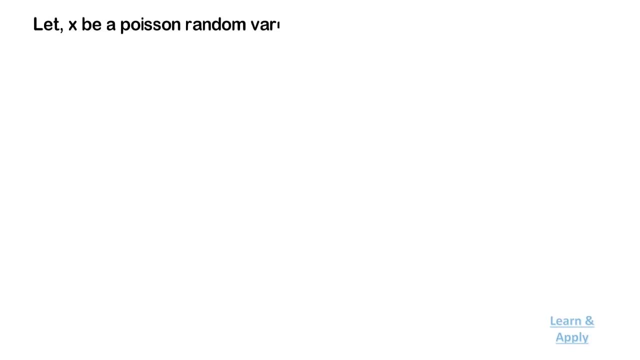 For the Poisson distribution, min is equal to number of occurrences per interval of time, which is denoted by λ, and standard deviation, which is equal to square root of min, which is equal to square root of λ. Let x be a Poisson random variable, then its probability, mass function, is probability. 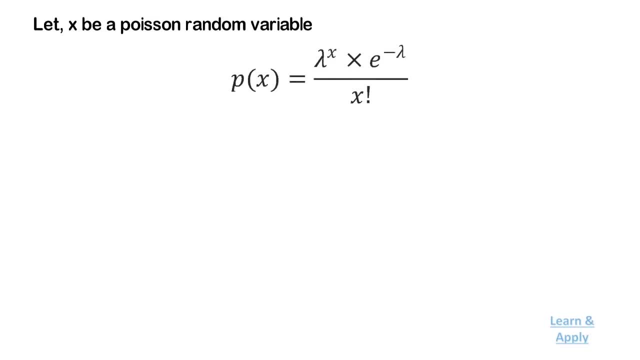 of x, which is equal to λ, raised to x into e, to the power minus λ whole divided by x factorial. For example, typos: The number of typographical errors in a big textbook is a Poisson distribution with a mean of 1.5 per 100 pages. 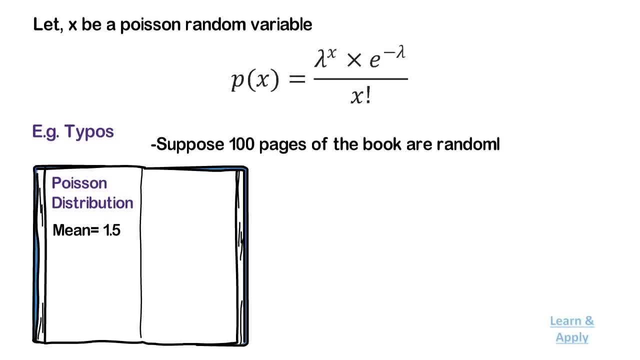 Suppose 100 pages. Suppose 100 pages. If 100 pages of the book are randomly selected, what is the probability that there are no typos Here? x is equal to 0 and λ is equal to 1.5, and probability of 0, which is equal to 1.5. 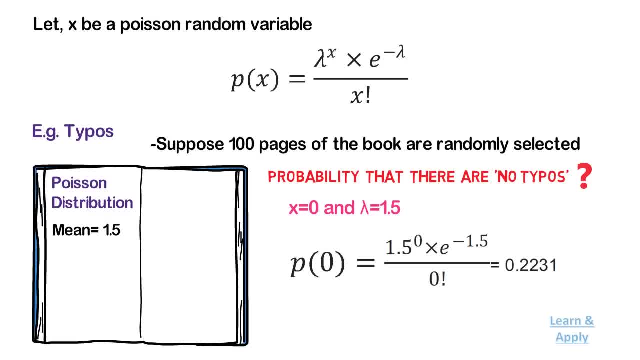 raised to 0, into e, to the power minus 1.5, whole divided by 0 factorial, which is equal to 0.2231.. That is, 22.31% is the probability that there will be no typos. 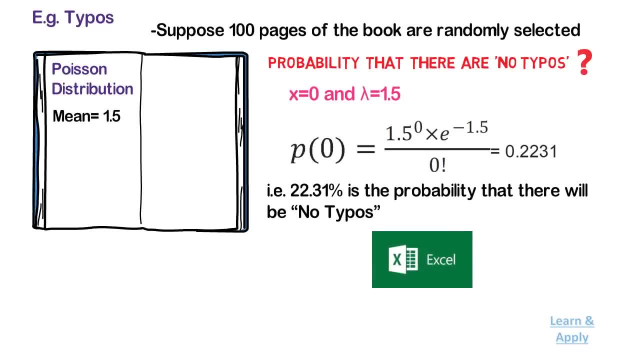 We can also use Excel To find probabilities related to Poisson distribution, random variable, the number of occurrences x in an interval and which is calculated at probability which is equal to Poisson x, λ and 0.. For the above example, probability of 0, which is equal to Poisson 0,, 1.5, and 0, which 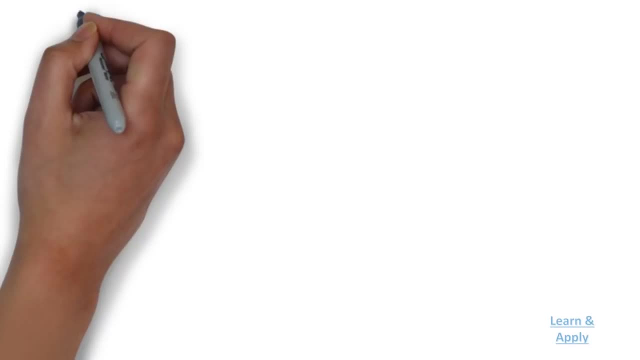 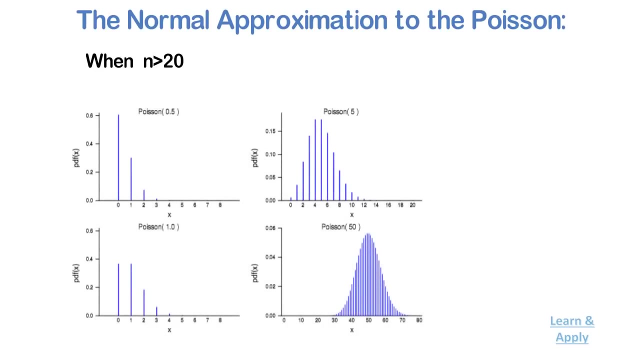 is equal to 0.2231.. The normal approximation to the Poisson When n is greater than 20.. When n is greater than 20. Or when the number of observations is very large, it has been statistically proven that the Poisson distribution becomes a very good approximation of the binomial distribution. 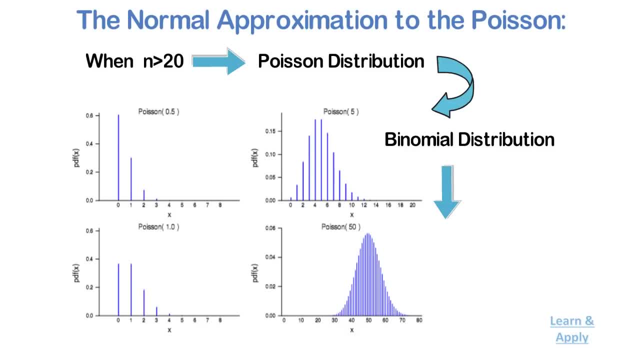 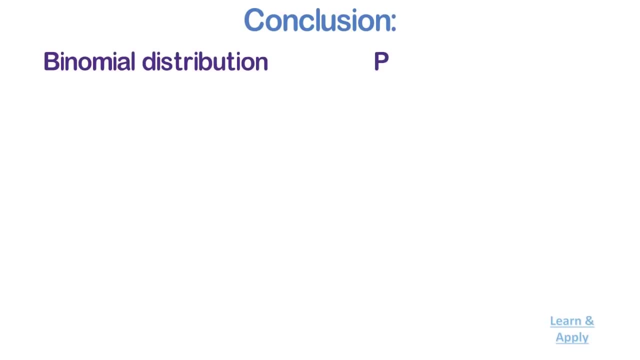 And, as seen earlier, the normal probability distribution is generally deemed a good approximation to the binomial probability distribution when np and n into 1-p are both greater than 5.. Conclusion: Both binomial distribution and Poisson distribution are used for discrete variables. 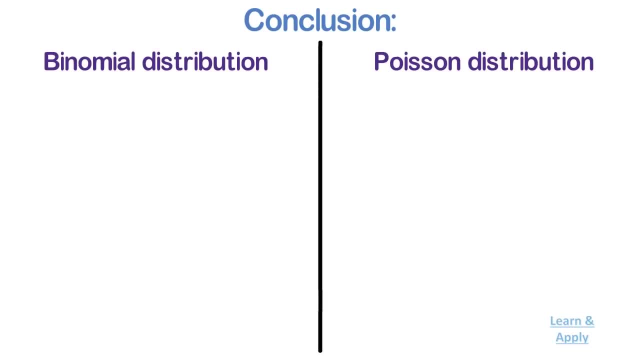 But there are some differences too. Let's see them one by one. 1. In binomial distribution there are only two possible outcomes, ie success or failure, whereas in Poisson distribution there can be unlimited number of possible outcomes. 2. 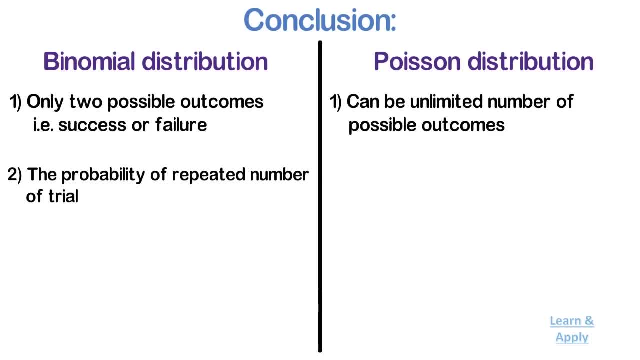 Binomial distribution is one in which the probability of repeated number of trials are studied. 3. Where, as 4. occur randomly with a given period of time. For example, experiment of tossing a coin and typo errors in a large book. In binomial distribution, mean is equal to. 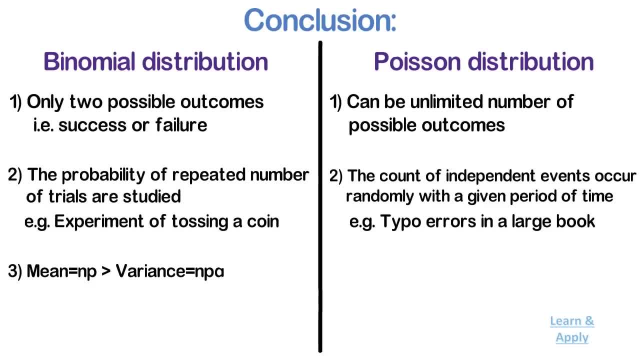 np and which is greater than variance which is equal to np cube, Whereas in Poisson distribution mean is equal to variance which is equal to lambda. And the last four binomial distribution has a constant probability of success, whereas Poisson has an infinitesimal chance of success. 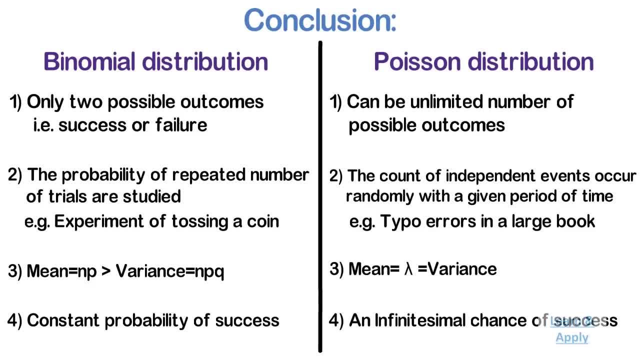 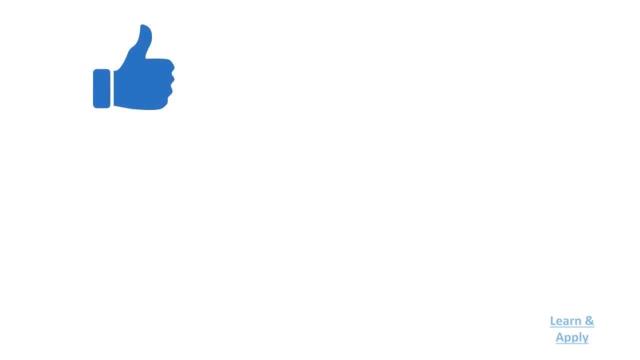 This is all about distribution for discrete variables. I will explain distribution of continuous variables in next video, and then we go for a MSI. Now to end, please like this video. if you have found it useful, Share this video to your friends and colleagues to improve and refresh their knowledge. If you want to get 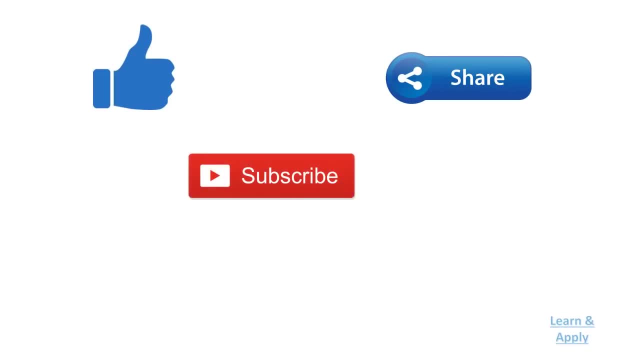 updates of such videos from my channel. please do not forget to subscribe my channel and click on the bell icon to get all the notifications. And finally, thank you for watching. See you in the next video.